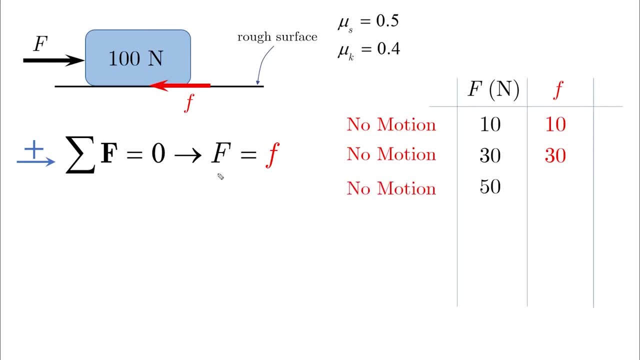 and no motion occurs. this means again that the friction force is in static equilibrium with the applied force. and then you notice that by increasing the force to just 50.1, the block starts to move, and now the static equilibrium is not valid anymore. we have to apply newton's second law, which is the summation of forces equals to ma. 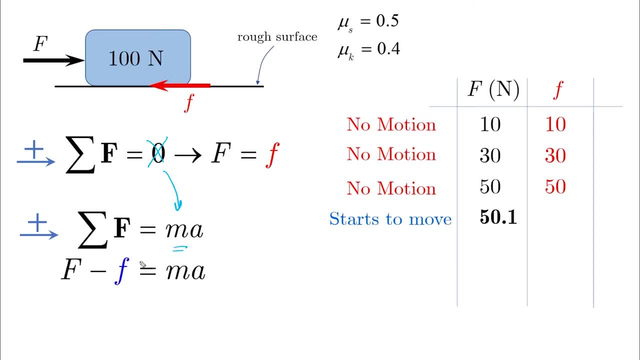 and now the applied force minus the friction force will be equal to m times a. however, you noticed also that the friction force dropped from 50 to 40 and when you increased the force applied to 80 newtons and the block moves faster, the friction force is still 40, even faster. 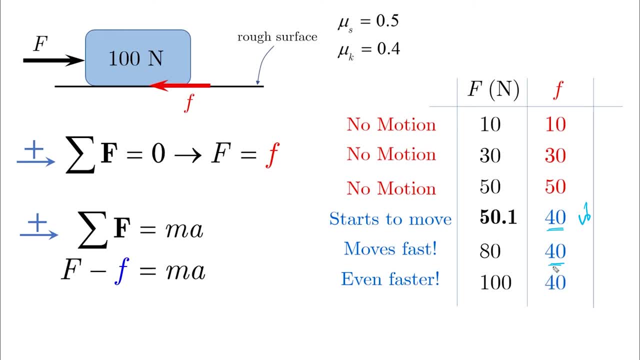 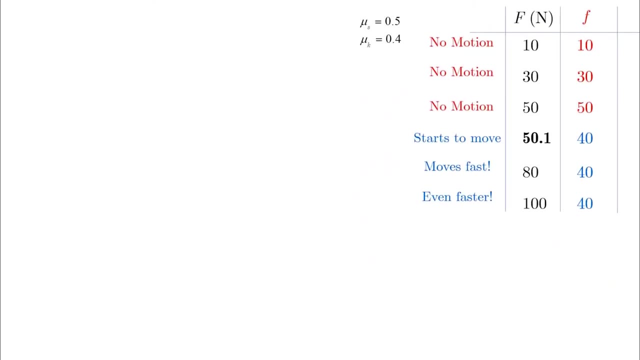 you will see that the friction force always have this constant value of 40 newtons. so what happened here that causes the friction force to drop and remains constant? and it's time to go behind the scenes to see what exactly and what physically happened. so this is our table. 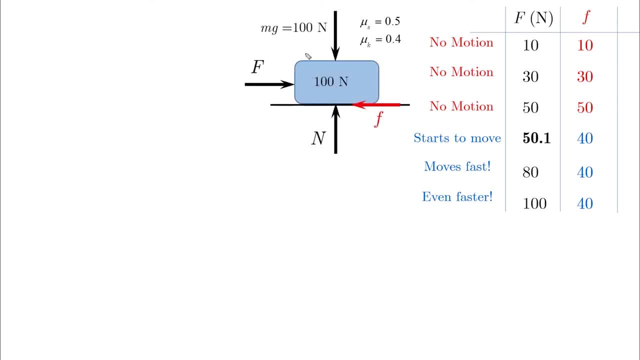 this is the free body diagram showing all the forces, and if we want to find the normal force, then we apply the summation forces, which is going to be equal to zero, and this leads to the normal force, which is equal to the weight or 100 newtons in this. 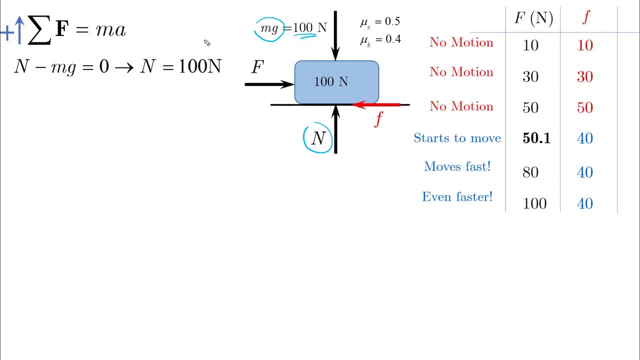 case, and by looking at our table, this is what is actually happening between the friction force and the applied force. so when we applied our first table- 10 newtons- we got 10 newtons of friction force. and when we applied 30, we got 30. 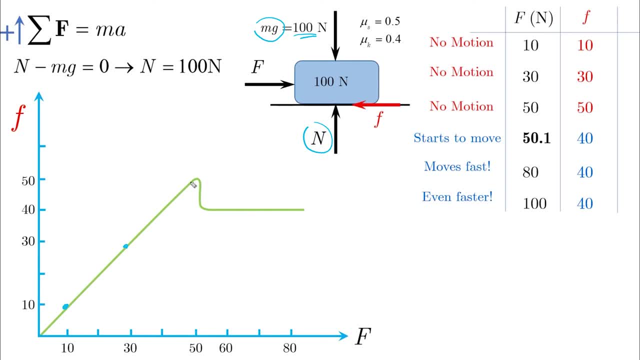 and when we applied 50, we got also 50. and in all these situations we are within the static friction region, which means there is no motion in this straight line. but at the top of this line we reached the so-called maximum static friction, which is equal to mu s times n. so you can see from here mu s is. 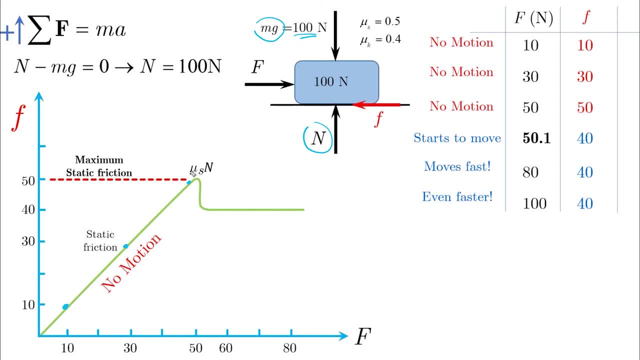 0.5 n is 100 and the maximum static friction is 50 newtons. so what happened when we increased the force to 50.1? now, 50.1 is larger than the maximum static friction, which is 50, and this means that. 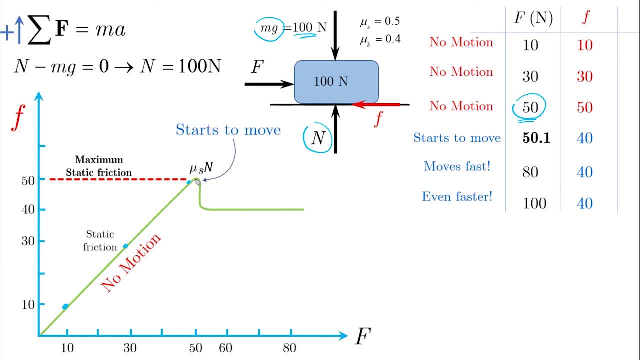 the block will start to move. and when the block started to move, the friction dropped because the kinetic friction is usually smaller than the static friction. so the kinetic friction now is mu k times n, which is 0.4 n times 100 or 40. and as long as we are moving, even if we increase the amount of 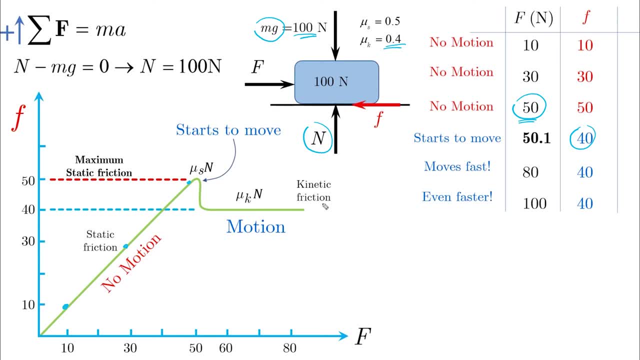 the force applied, the kinetic friction remains constant, always at 40 newtons or at mu k times n. so physically we have three situations. if the force or even other forces applied on the block are not enough to move the block, this means that the friction force is in static equilibrium with all. 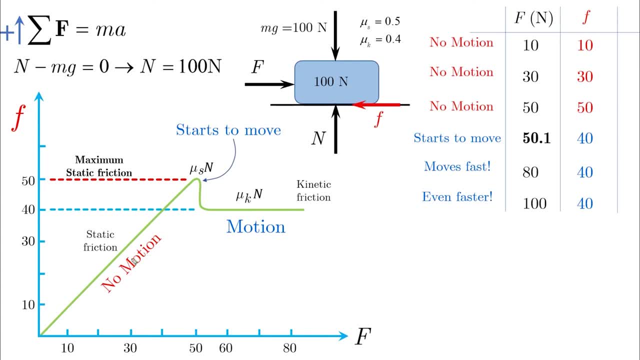 other forces and we can calculate its value from the summation force is equal to 0, and if the block starts to move, which is our second situation, the friction force is known. it is equal to the maximum static friction, which is mu s times n. and in the third situation, 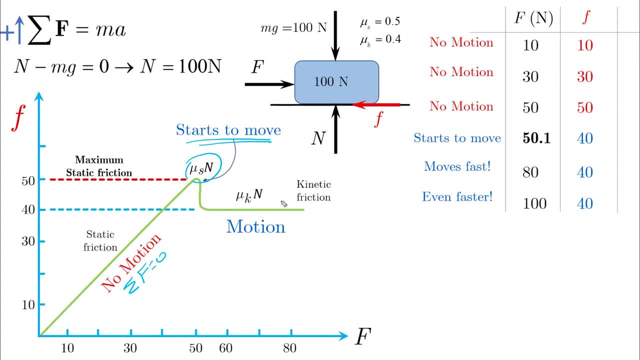 when the system is moving, with an acceleration for example, then the kinetic friction is applied, which is mu k times n. so again in the first region of the straight line no motion occurs. it's a static friction situation. so the summation force is equals to 0 and the friction force is unknown. we find it. 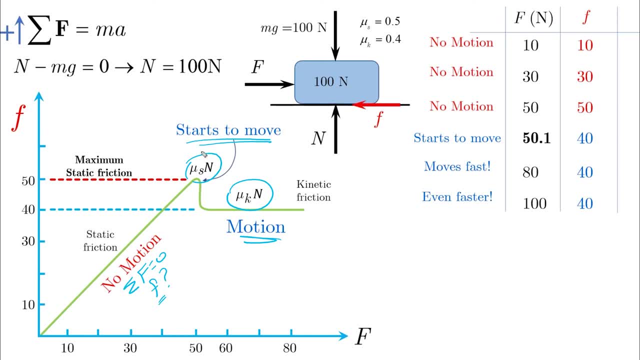 from the equilibrium, and the second situation, when the system starts to move. we have summation of forces equals to ma, with the friction force value known as mu s times n. and in the third situation, the summation force is equals to ma, with the friction force equals to mu k times n, because we have motion and we have 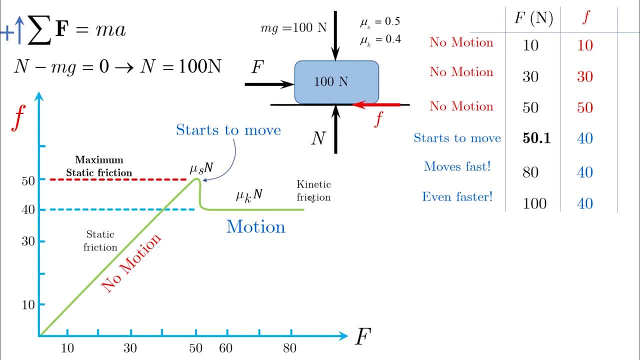 kinetic friction and finally, to put that in some useful mathematical relationships, we will say the following: if the friction is less than mu s times n, no motion is occurring. if the friction is equal to mu s times n, the system is about to move. and if the friction force is equal to mu k times n, this means 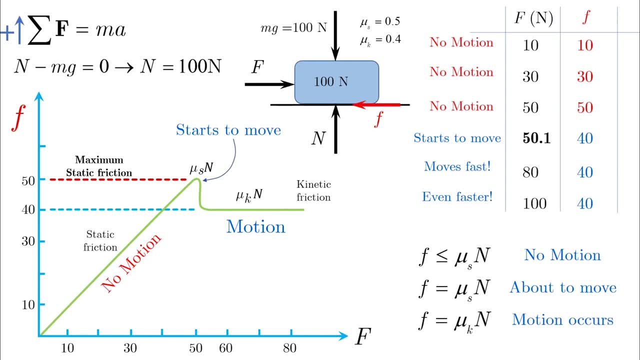 already that motion occurs and the system is moving. 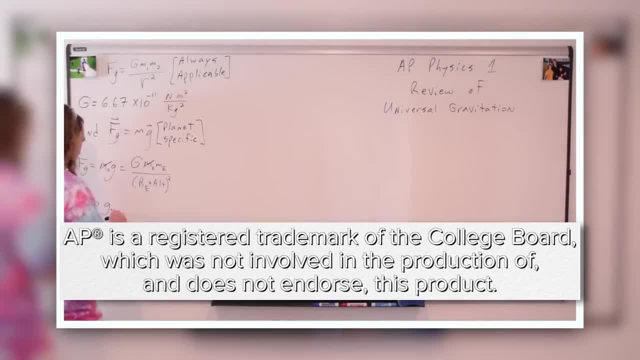 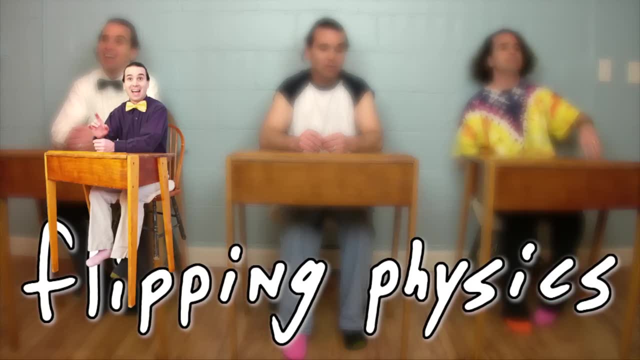 Mr, Good morning. Today we are going to review the universal gravitation topics covered on the AP Physics 1 exam. Hey guys, Hey Bo, Hi Bo, Flipping Physics, Mr. Let's start with Newton's Universal Law of Gravitation. 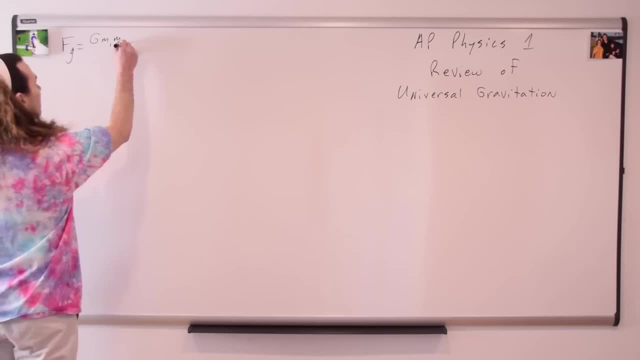 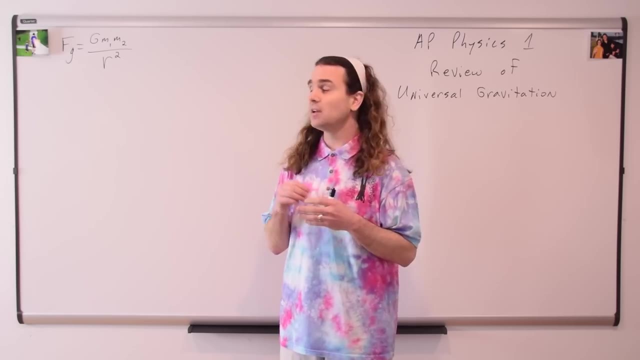 which I like to call the Big G equation. The force of gravity that exists between any two objects is equal to Big G, which is the universal gravitational constant times the mass of one object times the mass of the other object divided by r squared. 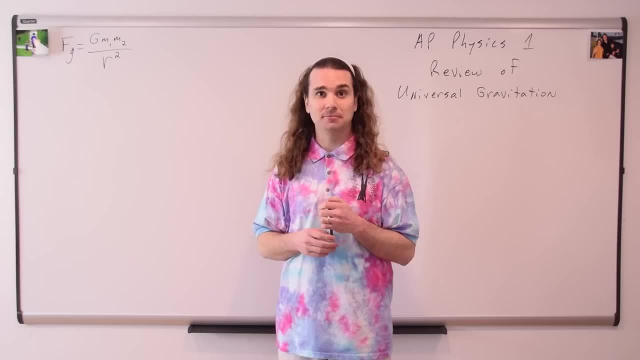 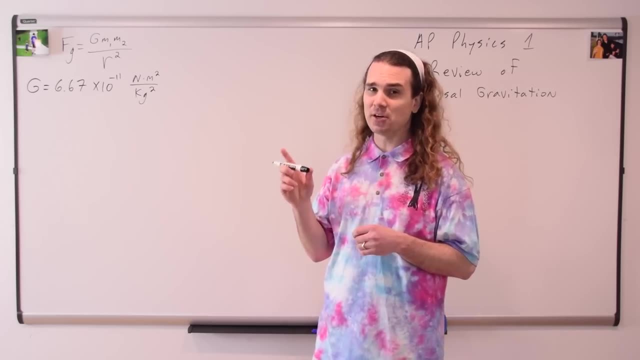 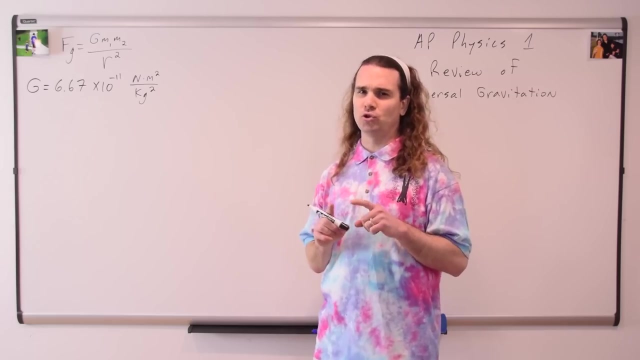 Where Big G is a constant and it is given as Big G is 6.67 times 10 to the negative 11 newtons times meters squared divided by kilograms squared, And n is the mass of the two objects in kilograms. It is r that usually gives students trouble.